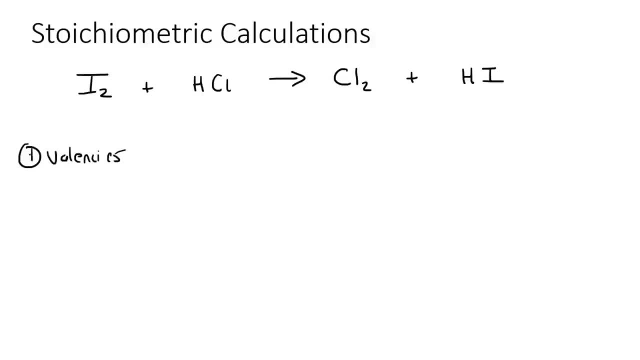 balance the valencies, which is the numbers that go on the inside, like over there. you know those kinds of numbers. and then the next thing you need to always make sure is balanced is the coefficients, Kevin. what are coefficients, bro? It's the numbers in the front. So let me quickly. 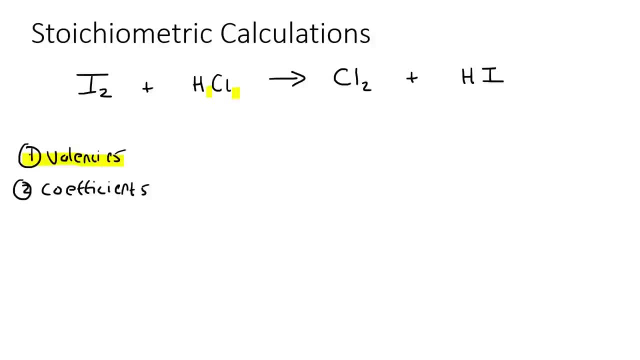 show you. So valencies are all the numbers on the inside. so there and there and then coefficients are all the numbers on the inside. So there and there and then coefficients are all the numbers in the front. okay, So we must make sure that all of that is balanced before we do any. 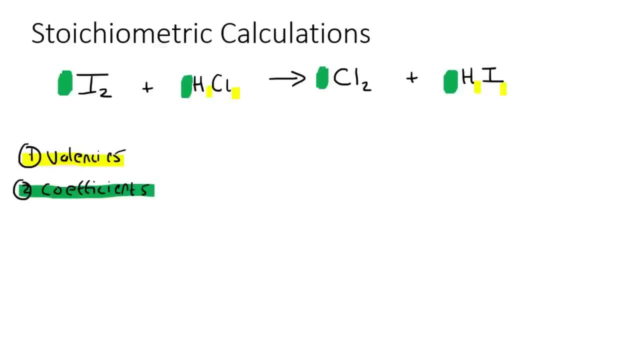 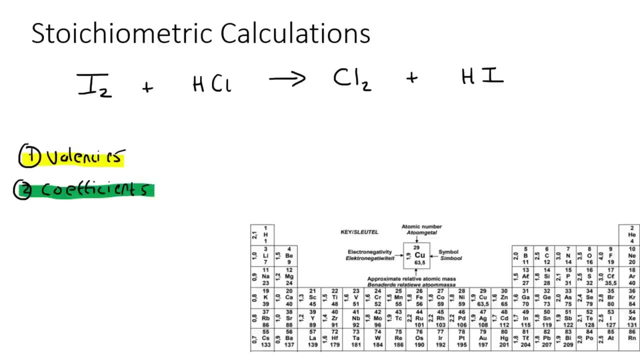 stoichiometry, Stoichiometry. we haven't even started that part yet. So to balance the valency numbers, we need to know the valencies from our periodic table And if there was anything like I don't know, something like NO3, SO4, those are polyatomic ions and those you would have to know. 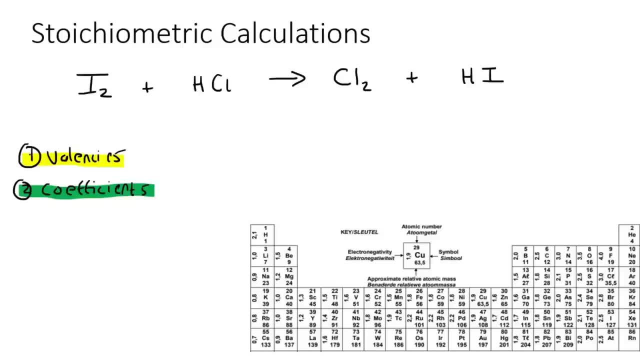 the valency by just memorizing from previous chapters. okay, So don't worry about anything. that's by the way, I'm going to show you how to do that. I'm going to show you how to do that by itself. We don't need to look at that Now. if we look at HCl, we know that hydrogen is in group. 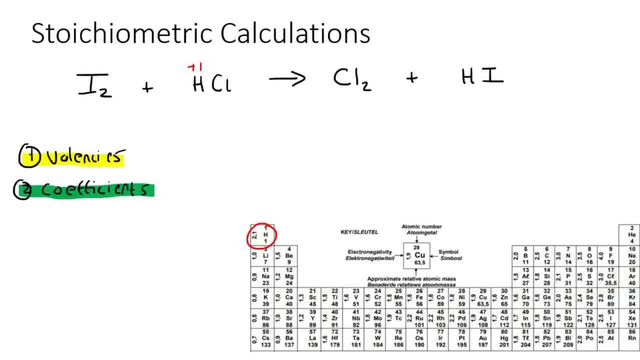 one, so that's a positive one for its valency. Cl is remember how valency goes: Plus one plus two, plus three, plus minus four, minus three minus two minus one. Now, oh, by the way, something I 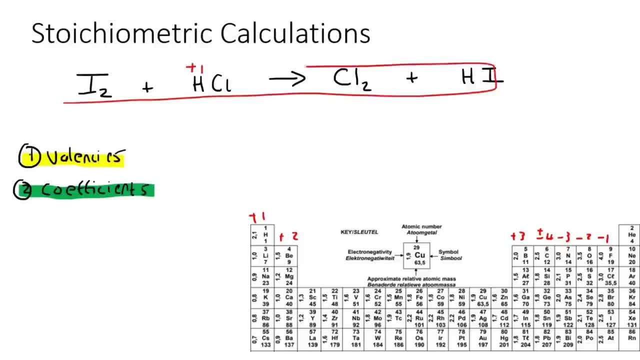 should mention. that's quite important. If they give you an equation like this, if they wrote out the whole equation, then the valencies would be balanced already. okay, But I'm just getting you into the technique of remember. I'm going to show you how to do that. So I'm going to show you. 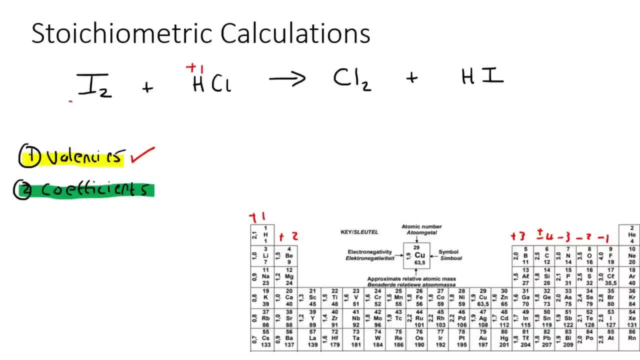 how to do valencies, because sometimes they're not going to give you the written equation like this, but they're going to write it out in words and then they're going to say something like hydrogen chloride, and then you need to go say HCl, but it might be HCl2, or it might be H2Cl. 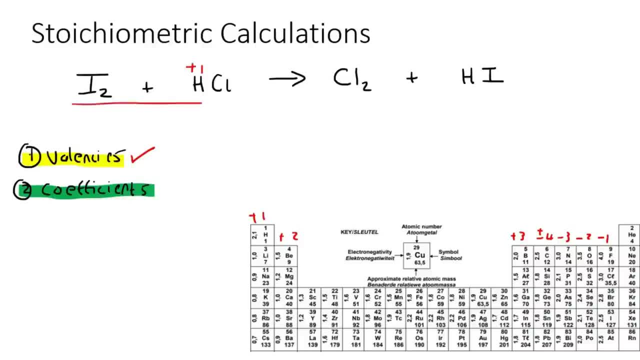 and those are the things. that's where it's important. okay, But when they give it to you written as a chemical formula like that, then the valencies are already done. but let's practice it anyways, okay. So Cl is negative. 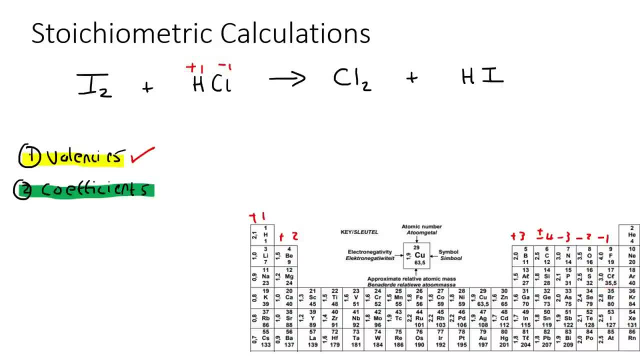 So when these two numbers are the same, nothing that you need to do. so that's all fine, Don't worry about anything. that's by itself. Now, for hydrogen, that's plus one. For iodine, that is negative one. So when these two numbers are equal, no worries about that. okay, So all the valencies. 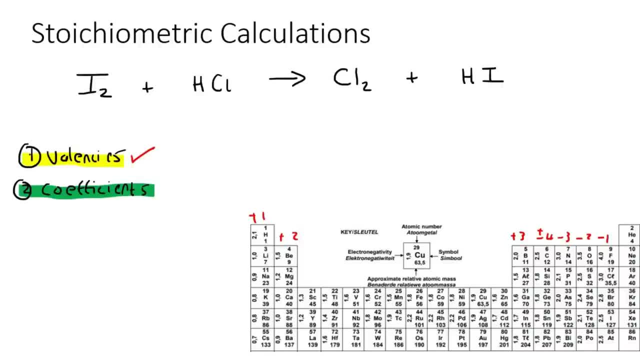 are done. We knew that already, but it's good to check and to practice that. Now the coefficients: Now to balance the coefficients, which is the numbers in the front, we use these steps that we looked at in one of our earlier chapters. 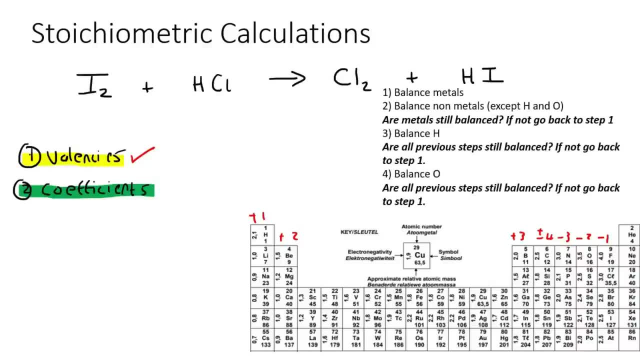 So step one: balance all of the metals. Now, in this example, there are no metals, okay, So step one is done. Step two: balance all of the non-metals. Now, remember, the non-metals are: 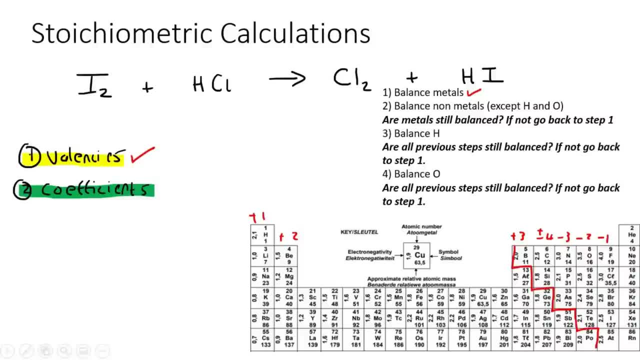 everything on the right-hand side of the step. but you can ignore: don't do hydrogen and don't do oxygen right now. That comes in later steps. okay, So any non-metals? yes, there's iodine and there is chlorine. okay, So we divide it into the left-hand side of the reaction. 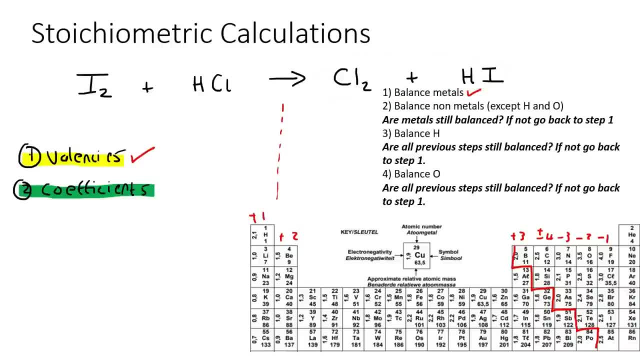 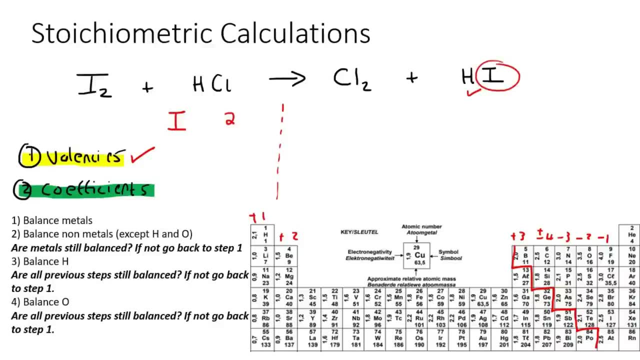 which is the left of the arrow, and the right-hand side of the reaction, which is the left of the arrow. So on the left-hand side for iodine there are two- At the moment there are two- and on the right-hand side there is only one. So to fix that you don't put a number over here, 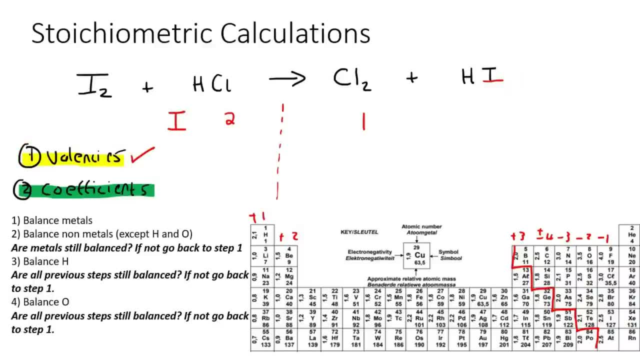 because that's a valency number and we've already done the valency numbers, So you have to put it in the front, okay, So now we have two on the left, two on the right. Excellent, Then the next. 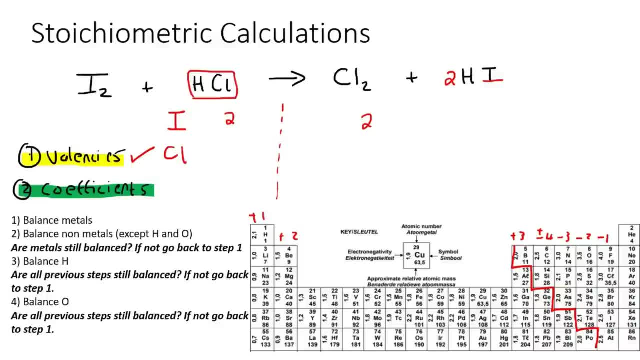 non-metal is chlorine. So on the left-hand side here we have one chlorine and on the right we have two. So we don't put a two here, you put a two in the front, Okay, So all the iodines and 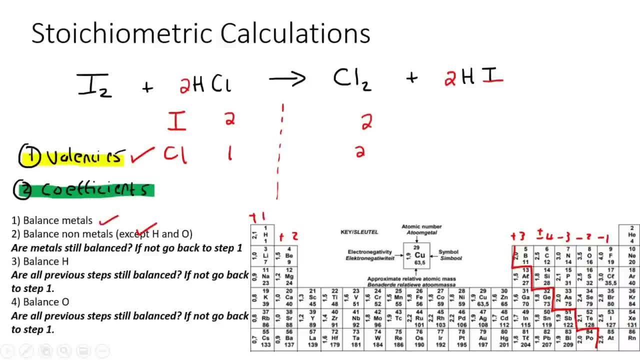 all the non-metals besides hydrogen and oxygen have been balanced. Next step: balance all of the hydrogens. So on the left we have two of them, and on the right-hand side we also have two, and then there's no oxygen. So we are balanced. Okay, guys, So now none of that. 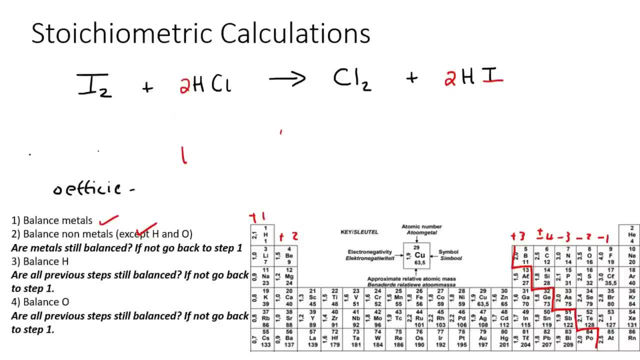 was stoichiometry, but that has to be done before we can do stoichiometry. To be able to do stoichiometry, the reaction must be balanced, Otherwise it just it's completely wrong. Now stoichiometry: the main thing I want you to think about in stoichiometry. 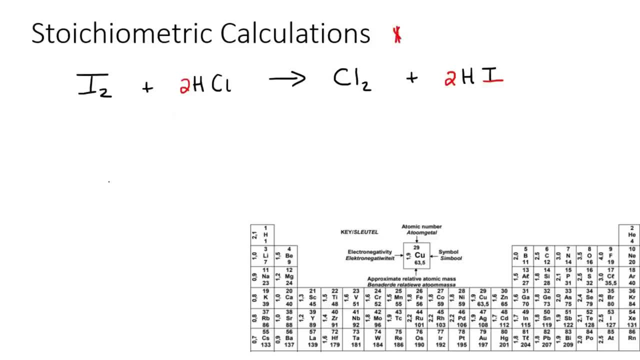 is the moles, Moles. Now, we've looked at a lot of different formulas in the previous lessons where we get moles. One of them was this one, Another one goes like this, Another one goes like this, And there's also one that uses concentration. Guys, these four formulas are golden in stoichiometry. 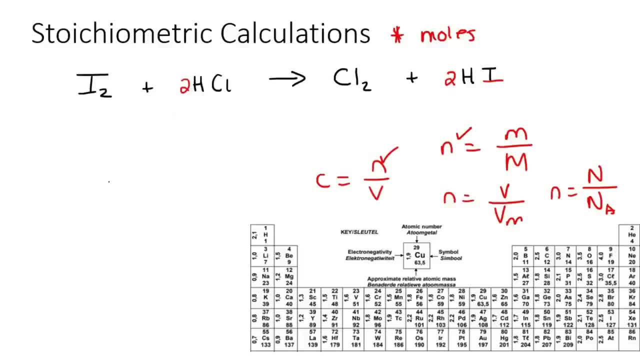 because each of them has moles There, there, there and there. So you are going to be able to, or you're going to need to know how to use all of them- and I have showed this in previous lessons- and you're going to need to know how to use all of these to be able to get moles. 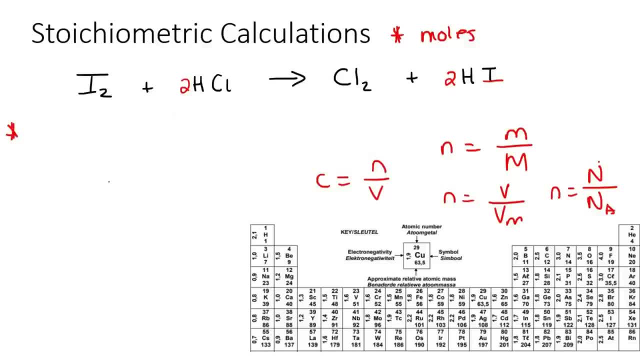 Because here's the golden rule of stoichiometry. If you or no, let me just say the golden rule is to get the moles of one of the substances. So if you could just get the moles of this one or this one, or this one or this one. 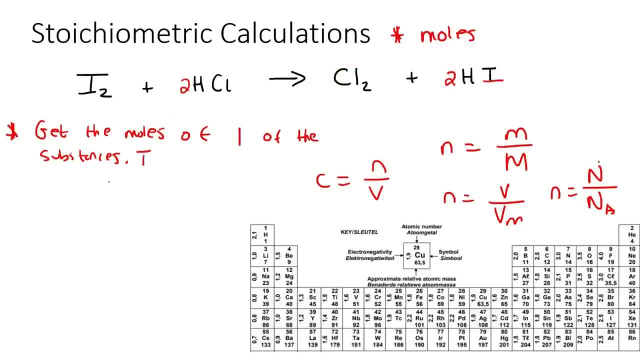 you only need to get the moles of one of them. then you will be able to calculate or to get the moles of all the others using ratios, And these numbers in the front are the ratios. Okay, So at the moment, this number is a one. this number is a one. 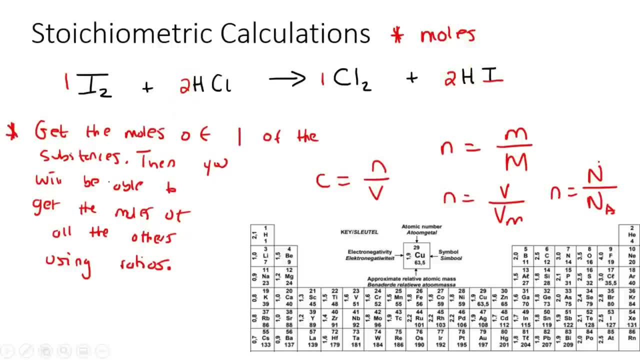 this number is a two. and this number is a two, So you only get the moles of one of them. and then you use the ratios to get the moles of one of them. So you only get the moles of one of. 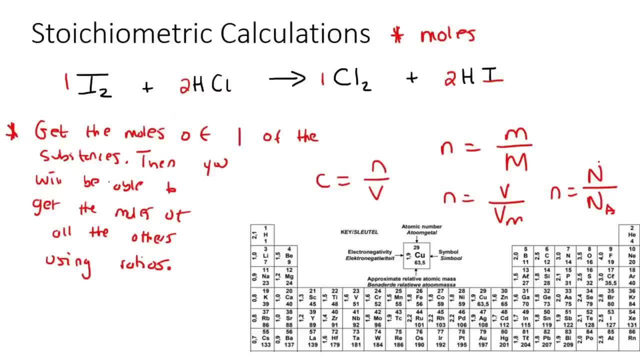 the moles of all of the others, And the way that you get the moles is depending on the information that they give you in the question. you would need to use one of these four formulas, Okay, so are you ready for that now? 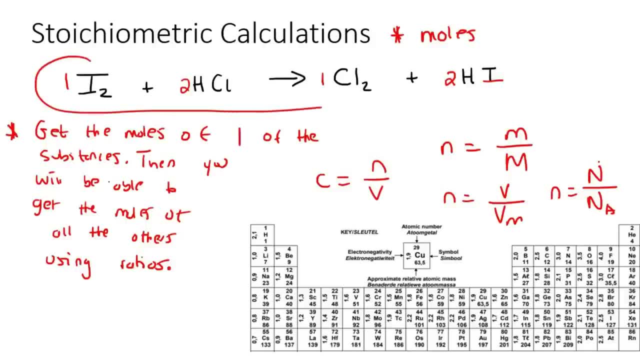 So I'm gonna give you some extra information about this question now, and then I'm gonna give you a question on that. So here we go. They tell us that 146 grams of HCl is given. Okay, so they tell us the mass of this one. 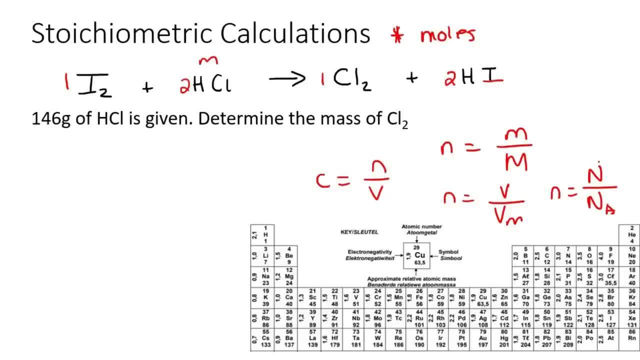 So we have this one's mass and then they say: determine the mass of Cl2.. So how do we go from there to there? Well, if you listen to what I said, I said: get moles. that's step one. So just go get the moles of this one. 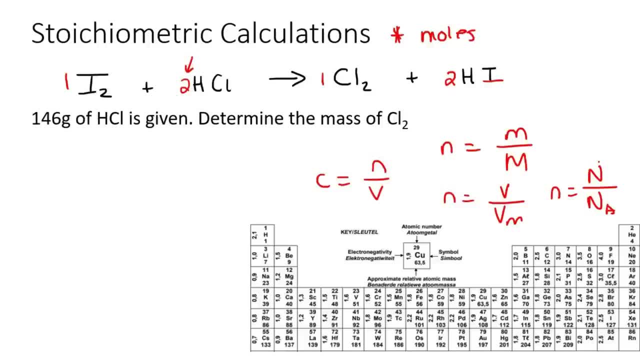 Now be careful. A lot of learners get confused with what to do with this number in the front. So they've given us the mass of HCl. So we're gonna use this formula. So we're gonna say N equals to M over capital M. 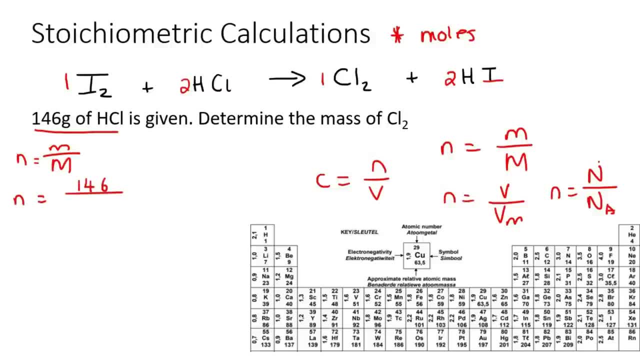 And we're gonna say the given mass is 146 grams of HCl And the mass on the periodic table- remember this capital M is called molar mass on the periodic table and it's got one hydrogen and then there's one chlorine. 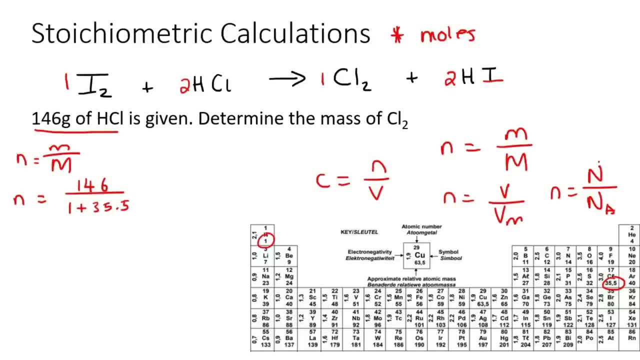 so that's 35.5.. Okay, so if you had to work that out, you end up with four moles. So I'm just gonna say here four mole. So that means we have four mole of HCl. But, Kevin, what is the two in the front? 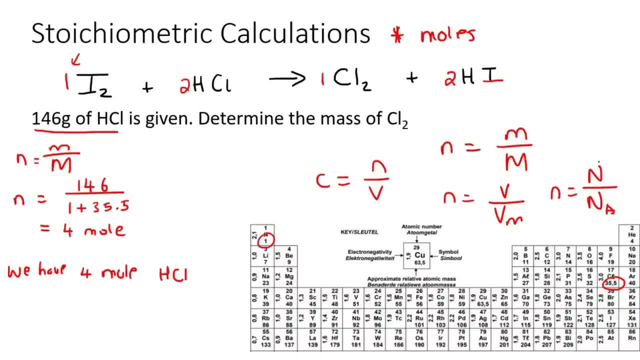 Doesn't the two mean we have two moles? No, not at all. These numbers in the front are just ratio numbers. okay, They have nothing to do with how many moles we have. Okay, so there, we've got the moles of one of them. 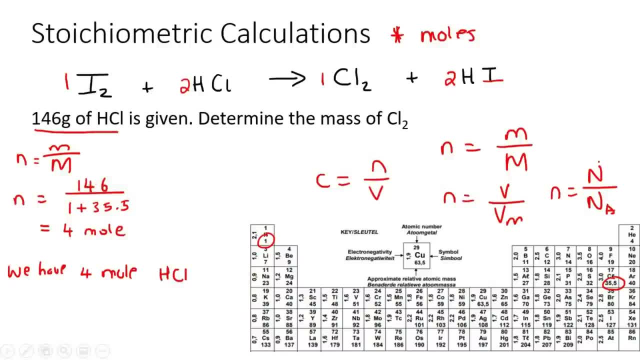 Now remember what I told you over here. I wrote a little thing down. I said: get the moles of one of them. So once you've done that, everything is easier, or everything's easy from the step onwards, okay. 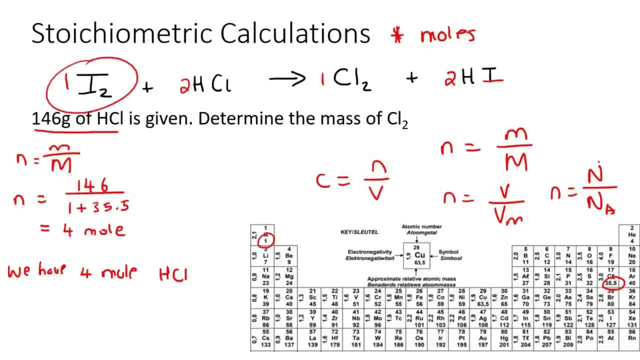 Because now we can go get all of the moles for this one, this one and this one, just using ratios, But we don't need to go get the moles of this one or this one because they're not asking us about those. 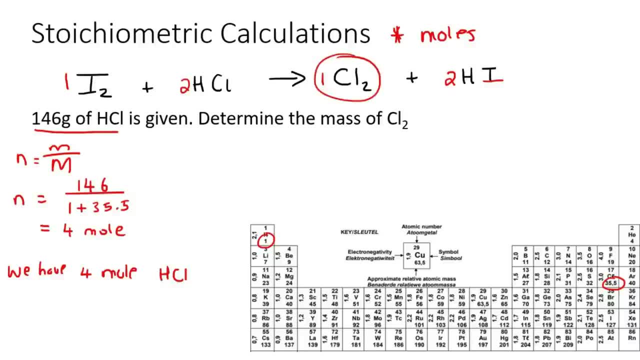 They're only asking us about this one. So here's where ratios come in, and this is why it's important that we balance the equation first. So if you look at the ratio of HCl to Cl2, the ratio over here is two to one. okay. 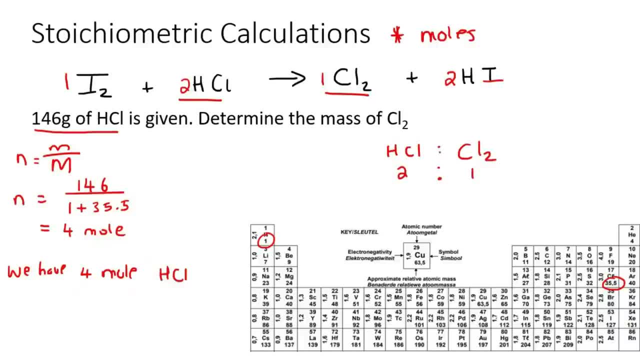 What you then do is you take what we've worked out, which is HCl, and we have a four, But what we don't know is that HCl is two to one. So what we know is what this would be okay. 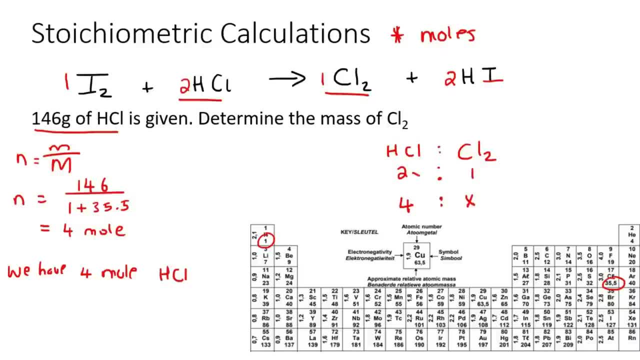 So that's a X. So what you now do is you connect these two using arrows. Don't worry, this is all gonna become clear as we do more examples. Right now, it is gonna feel a bit weird And what you're gonna do is you're gonna multiply the arrows. 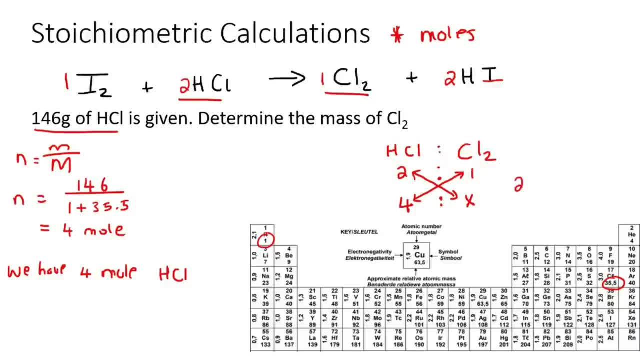 So you're gonna multiply those two, So that's gonna give you two X. you say equals, and then you're gonna multiply these two and that'll give you four. Then I want you to solve for X, So X would be four to one. 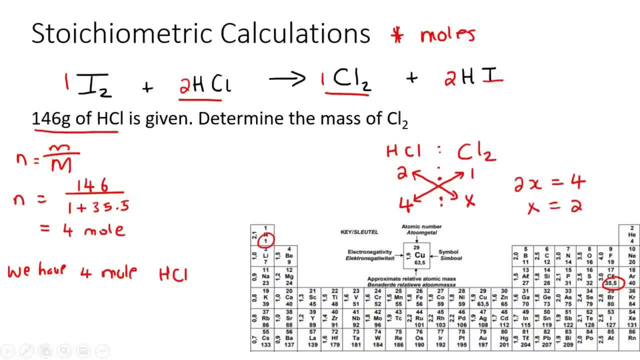 Four divided by two, which is two. So that means we have two moles of Cl2,. okay, So therefore we have two mole of Cl2.. Now that we know the moles of Cl2, we could use this formula again: 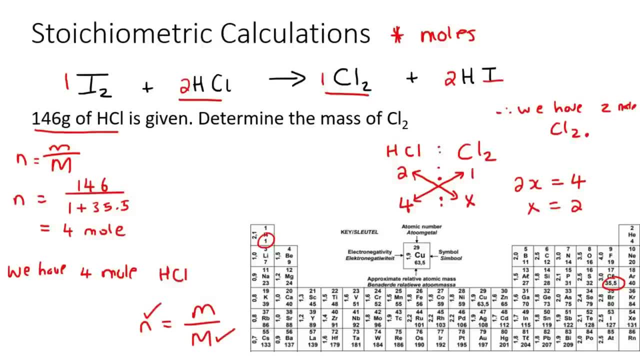 because now we have the moles of Cl2, and we also know the mass of Cl2 on the periodic table, and so that will allow us to work out the mass, And that is what they've asked us to do. So remember that to be able to get this one, 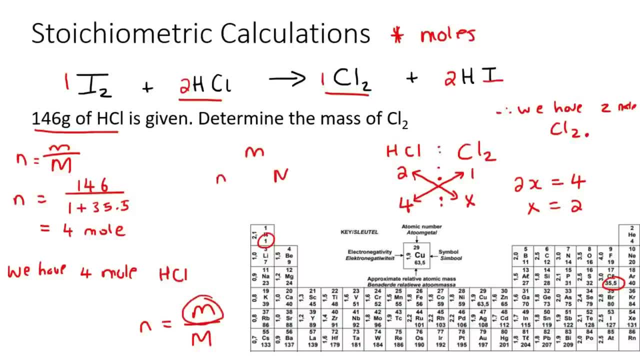 you could make a little triangle for yourself, which we've looked at before, okay, And to get this M at the top, you end up saying N multiplied by capital M, And so to work out the mass, we'll take the number of moles which we have, two. 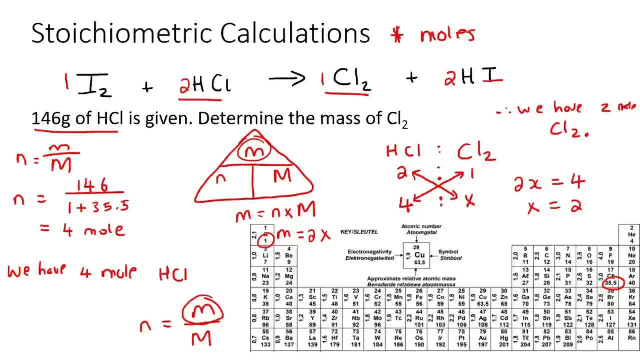 multiplied by the mass of Cl2 on the periodic table Now Cl2,, there are two chlorines. So you never, ever use these numbers in the front on the periodic table, never, ever, ever okay, But you do use the numbers on the inside. 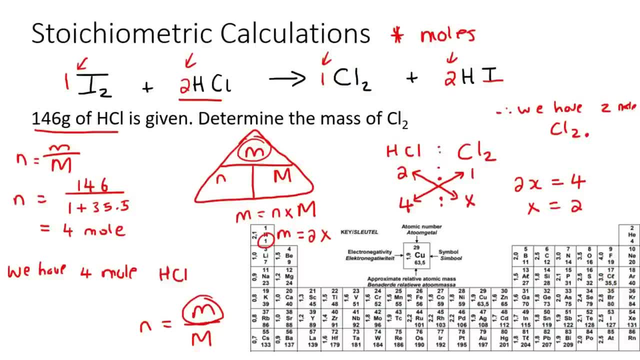 So Cl2, there's two of them, so that's gonna be 35.5 times two, And so if you had to go calculate this, you end up with 142 grams. 142 grams- let's rather write it over there. 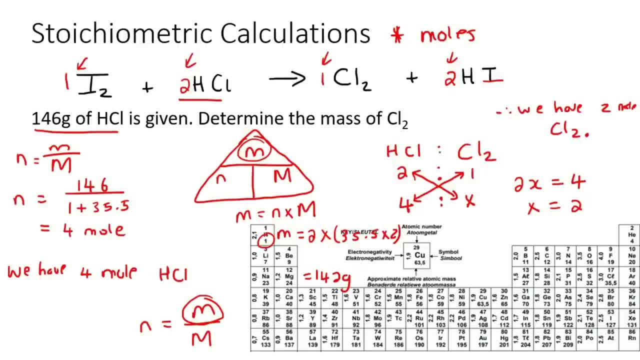 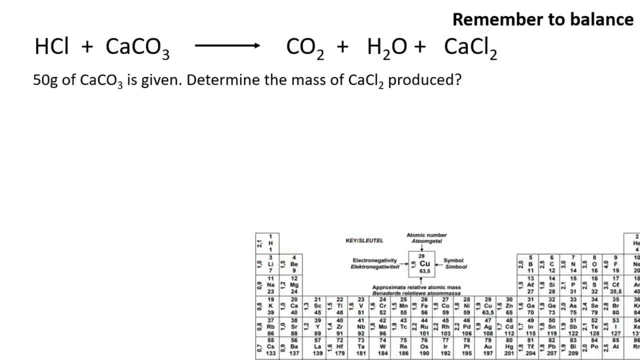 And that would be the answer of that question. okay, But now we need to do a lot more, because I know right now you might still be feeling a bit weird about all of this, so let's go do some more examples now. All right, so here's our next example. Now, remember first step, remember. you need to. 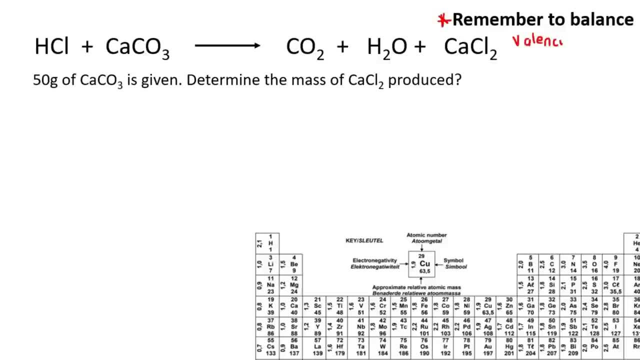 balance. Now, there's two things you always need to check, and that's the valencies. but we are going to skip that step because I told you in the previous example that when they give you the equation, the valencies are balanced. You know the little numbers that go in the inside. they would 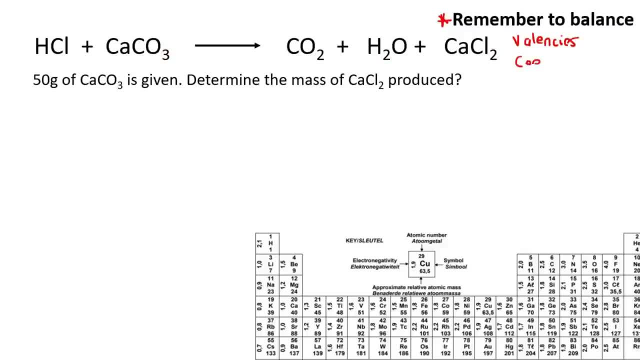 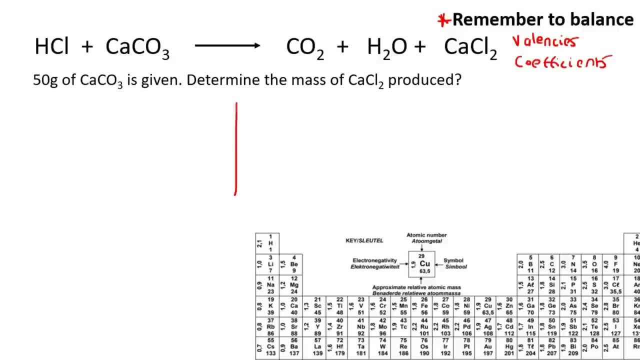 at this part. Okay, so let's go balance. So remember, here's the steps that we follow when balancing an equation. So we always start with metals. Now, metals are the things on the left-hand side of this line. Obviously, hydrogen is actually. 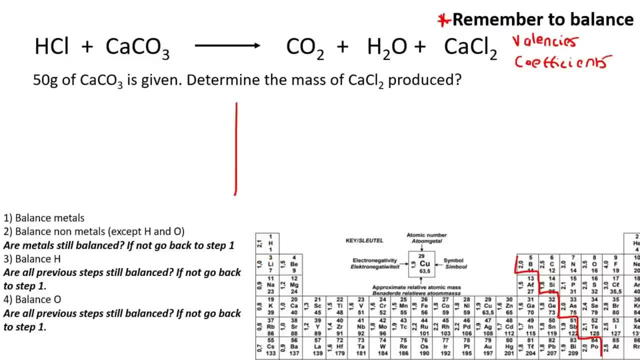 a non-metal. So the non-metal- I mean the metals that we have- would be calcium- See calcium over there. So on the left-hand side we have one calcium and on the right we have one calcium. The next step is to go balance all of the non-metals, except if you have hydrogen and 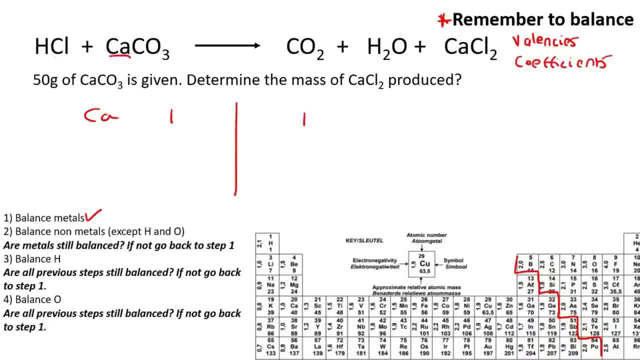 oxygen. So, like, don't, don't do those. So the only non-metals we have would be chlorine, because it's over here on the periodic table, and carbon, which is over here. So let's go do chlorine. So chlorine. on the left we have one. 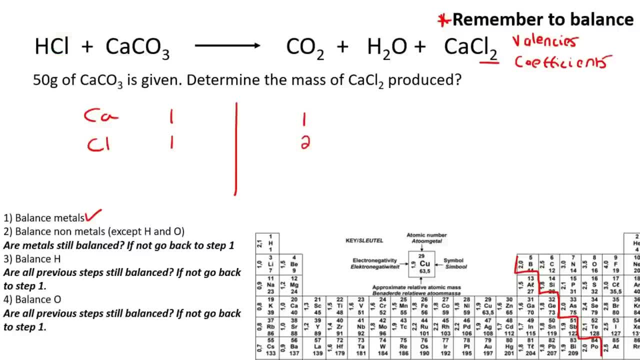 And on the right we have two. So to balance that, you don't put a two here, you put it in the front. Okay, so now we have two chlorines on the left, two chlorines on the right. Now we're going to go look at carbon. So on the left-hand side we have one carbon And on the 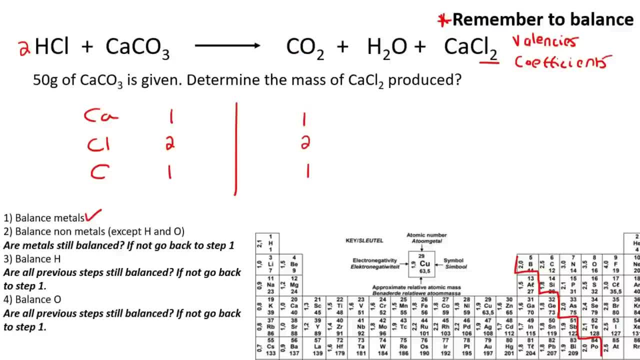 right-hand side, we also have one, carbon. Okay, so all the non-metals are done. Now we move on to hydrogen. So on the left side we have two hydrogens, we also have two. that looks good. then we go to oxygen. lastly, and on the left side, we have three, 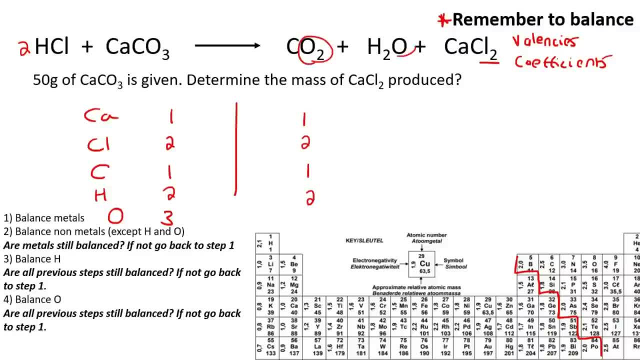 so three oxygens, and on the right we have two plus one, which is three, and so everything is now balanced. so now we can actually start the question and remember it's all about moles, so always keep that in mind, and there are four different formulas that we have. 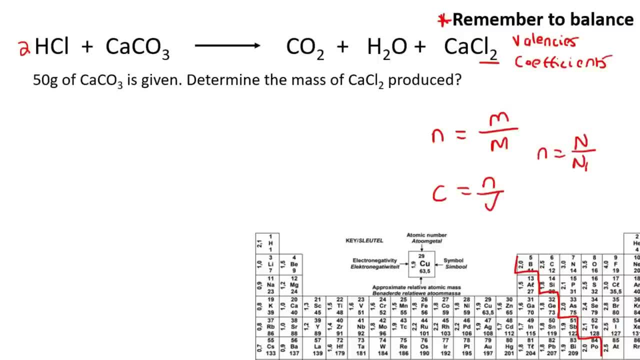 that use moles and you are going to use the one depending on what information they have given us. so here, they gave us 50 grams. okay, so we're going to use this one. so we're going to use n equals to m over capital m, and our goal is to try get the moles of any one of these. so let's. 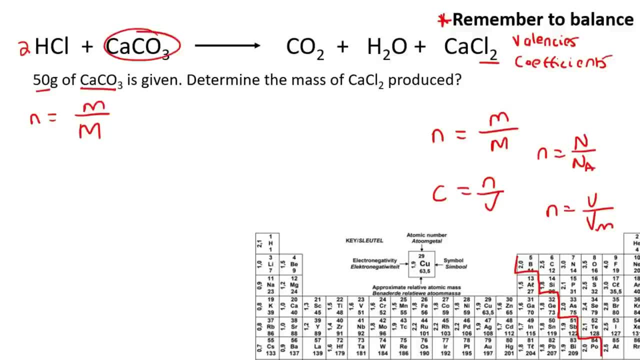 see what they've told us. they said 50 grams of caco3. okay, so we can get the moles of this one. so we're going to say 50 over now to work out the mass of caco3, the molar mass. you go to the. 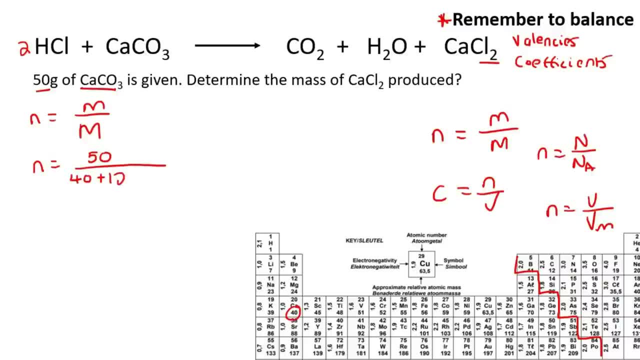 periodic table. so there's a, so there's a, so there's a calcium, there is a carbon and there's three oxygens, three times 16.. if you had to go calculate this, you should end up with 0.5 mole. so we have the moles of caco3. the moles of caco3 is 0.5. 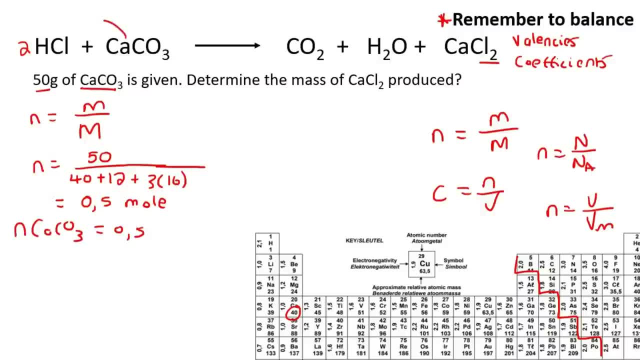 now. with that, you could get the moles of this one, this one, this one and this one, but we don't have to go get all of them. we now need to read the question. it says: determine the mass of of cacl2. okay, so we're going to get the moles of cacl2. so you need to look at the ratios, look at the 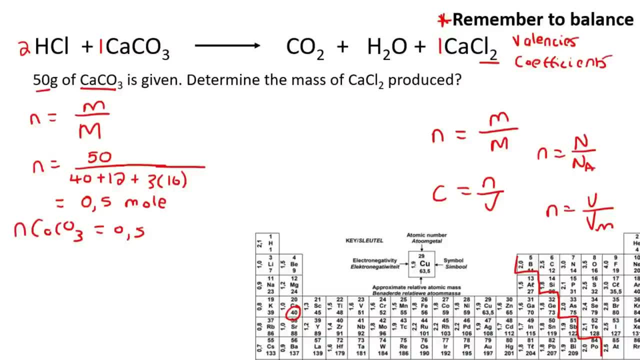 number in the front, one and one ah. so their ratios are the same. so that means this number is going to be the same. but let me show you how we do that. so you put caco3, then you put cacl2 and then you put the ratio that you see in the equation. then you put what we have and then you work out x. 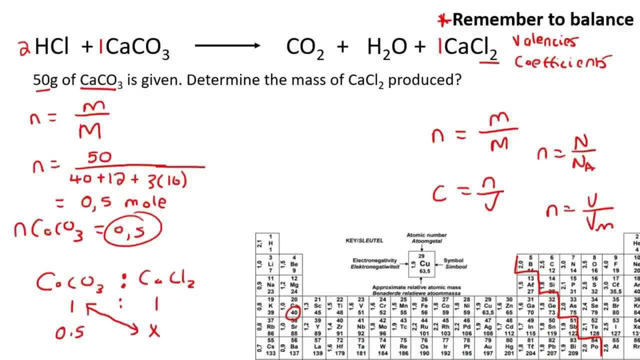 so here's where you do the arrows. so those two and those two. so you're going to multiply these two and that'll give you 1x. then you're going to multiply these two and that'll give you 0.5, and so if you calculate x, you're just going to end up with 0.5. so that means we have. 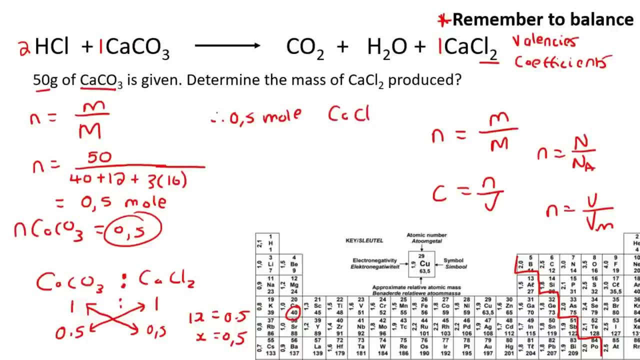 0.5 moles of cacl2. so now they asked us to find the mass of cacl2 so we could use this formula again: n equals to m over capital m. and so you could say: now remember, when you want to get this one, then your formula changes to this: okay, and so the number of moles. 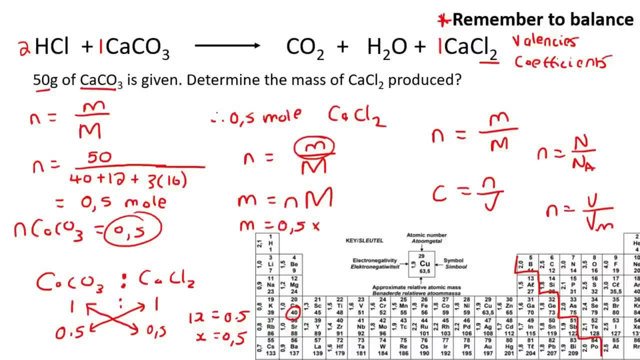 is 0.5. now the mass of cacl2 is going to be. there's one ca, which is 40, and then there's two cl molecules. so 2 multiplied by 35.5, and if we had to go calculate this, we end up with 55.5 grams. 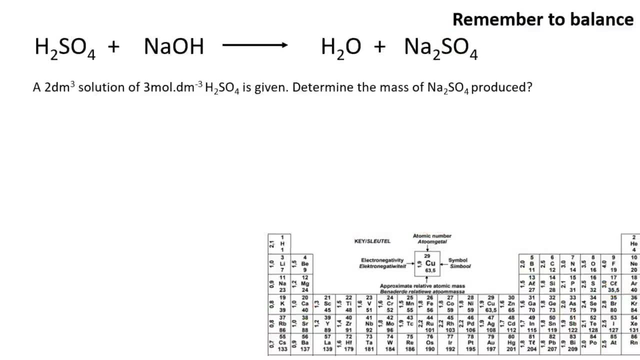 so here's our next equation: now remember. our next question. now the remember: the important thing is that you always balance this first. okay, so the way we balance is we use these steps over here, so we divide our reaction into a left side and a right hand side. 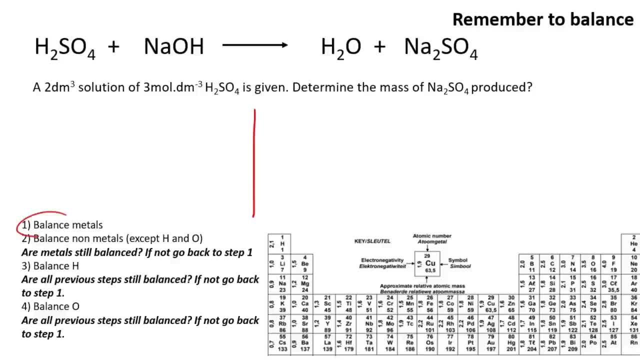 and we're talking about the left and right of this arrow. so we start by balancing metals. now, metals are everything to the left of this jagged line. okay, so your metals would be na. for example, hydrogen is not a metal, it's. you've got to remember that hydrogen actually is a non-metal. 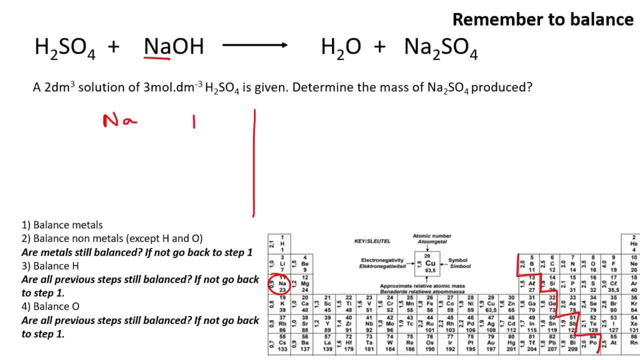 so on the left hand side we have one na on the right hand side we have two. so we fix that now by not putting a two there. those are valency numbers. we don't change those. we put a two in the front because that two is says that there's two nas, two oxygens, and 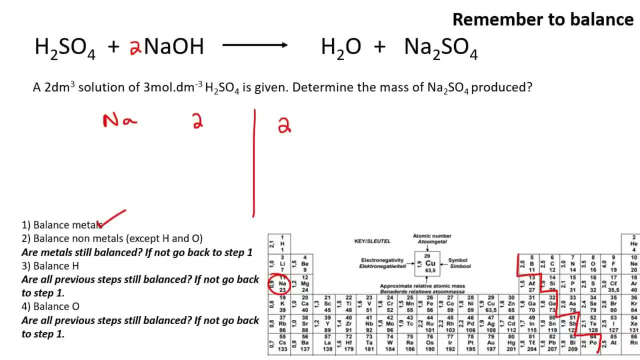 two hydrogens. so now, on the left we have two. now we go to the next step, which says balance: all of the non-metals, which is everything on the right hand side here, except for hydrogen and oxygen, so that would be sulfur. on the left we have one, and on the right we also have one, so that's. 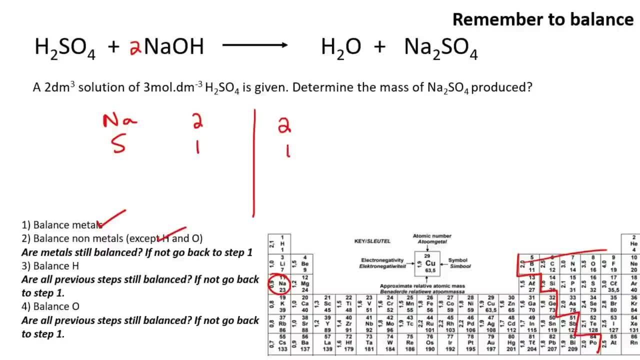 balanced. now we can go to hydrogen. so on the left hand side we've got two over there and then another two over here, because, remember, this two is for all of those, so that's going to be a total of four. now on the right hand side we only have two, so i'll put a two over there. so that makes four. 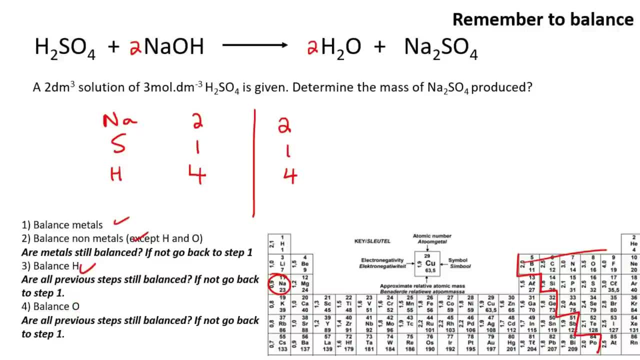 hydrogens. we're now going to do oxygen. so on the left hand side we have four over there and another two over here, because- remember, this two is for all of those- that's going to be six oxygens on the. that's a total of six oxygens, so our equation is balanced. only now should we go and do this. 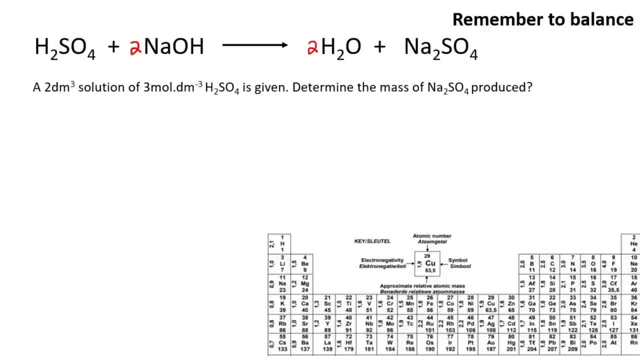 question. so we have learned that with stoichiometry it's all about getting the moles, and you just need to get the mole of one of these substances and then from there you can get the moles of any of the others. so remember, there are four different formulas based upon, or four different formulas. 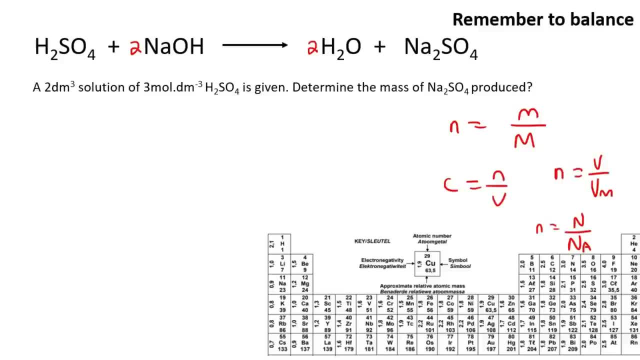 that you can use, depending on what they give you. so there we go. so here they give us a volume. okay, now you might be thinking, oh, okay, so maybe i should use this one. but this formula only gets used when they mention that there's a gas. so one of these would have to be a gas, and they 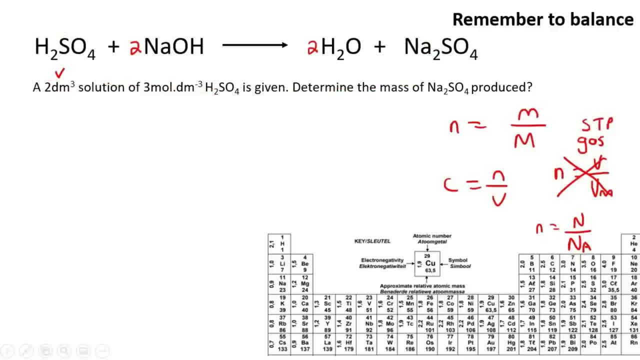 would usually use the word stp, which stands for standard temperature and pressure, instead we are actually going to use this one. now. the reason is is, if you look here we've got a mole, dot dm minus three, that is concentration. so they've given us concentration and volume, so we could use this. 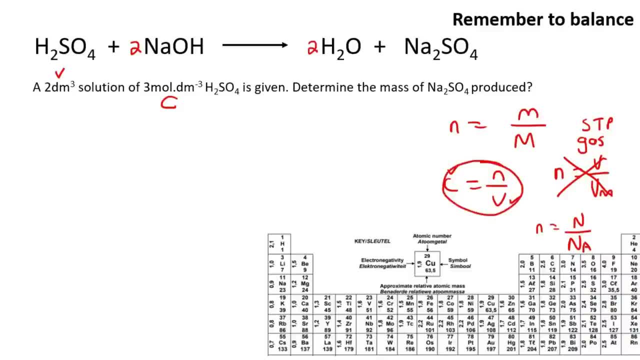 formula and we're going to use this one, and we're going to use this one and we're going to use this formula to get moles. Now make sure that you use this formula in the correct way, So you see how the moles is at the top, so you could make a little triangle, or let's actually do that down here. 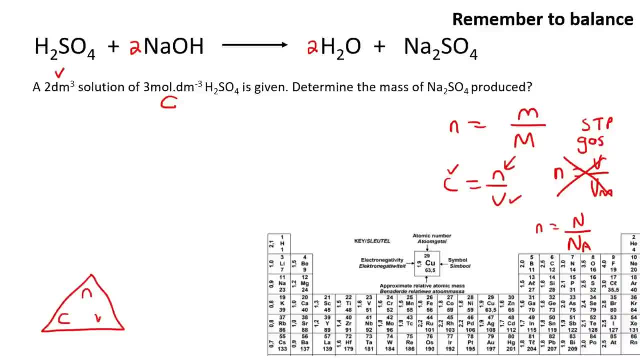 where the n would be at the top, and then you would have a c and a v. So if we had to, because the n is at the top, you would just multiply these two, because they're next to each other, so it's just c times v, and so we could say here that n is equal to c times v. So they tell us that we have two. 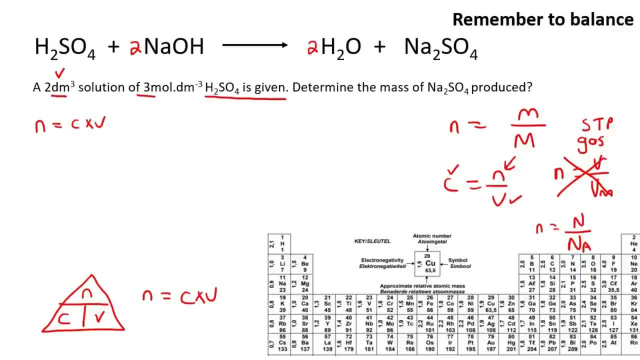 decimeters and three mole per decimeter of H2SO4.. So we could work out the moles of H2SO4.. So I'm just going to say here: moles of H2SO4 is equal to the concentration, which is three multiplied by. 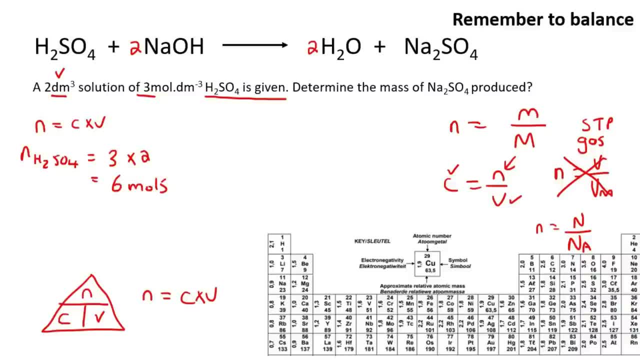 the volume, which is two, and that's going to give us six moles. Excellent, That is the most important part, because once you have the moles of one of these, then you can get the moles of any of the others, depending on what the question asks. So the question says: determine the mass. 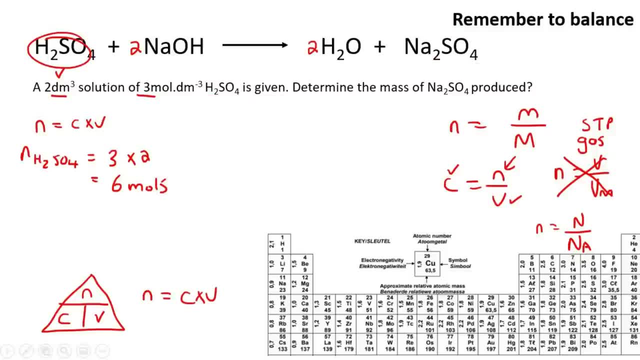 of the moles of H2SO4.. So if you have the moles of one of these, then you can get the moles of this that is produced. Okay, so if you look at the ratios, the number in the front, there's a one there. 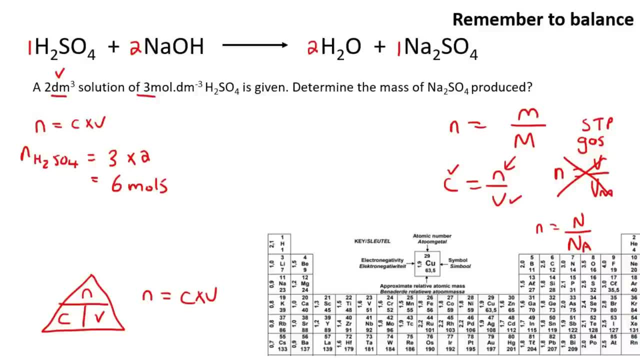 and there would be a one there. So they are equal. So you could say H2SO4 to Na2SO4, they are equal one to one. So if we have six moles of H2SO4, then you could go do the calculation. but 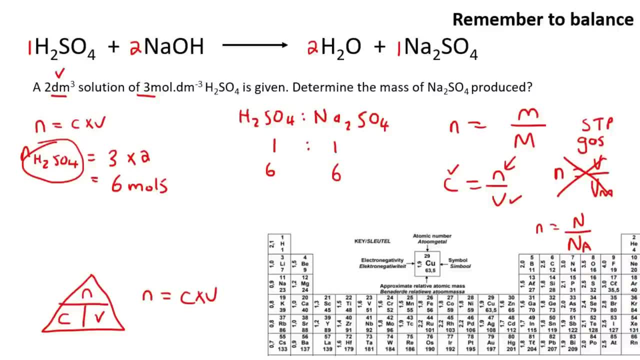 that means you would also have six moles of Na2SO4, because one is to one is the same as six is to six. So we have six moles of Na2SO4.. So the moles of Na2SO4 is going to be six. Now they want us to find the mass, so we could now use this formula over here. 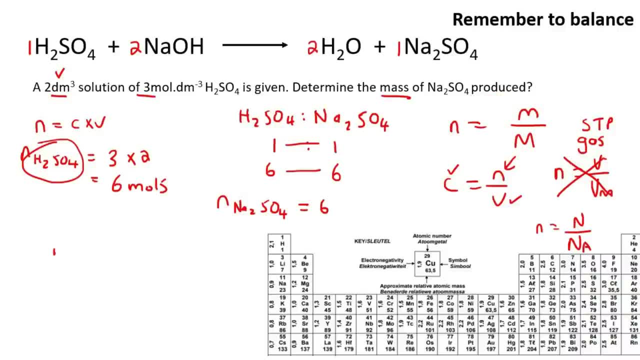 So if you had to make that into a triangle, this one's at the top, so it would be like that and then like that, and then like that. Oops, sometimes all my triangles came out so ugly. Okay, there we go too bad, okay. so if you're trying to calculate this m over here, you would say m is equal to. 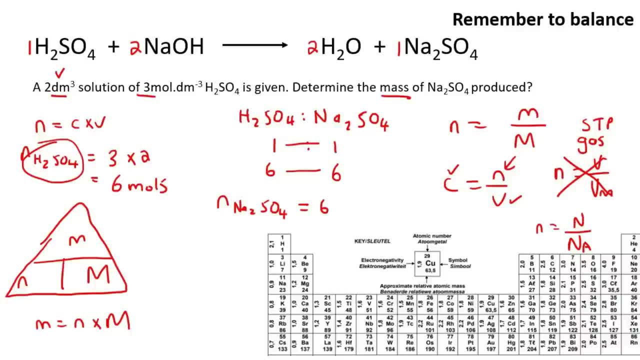 n multiplied by capital m, and so the mass would be equal to the number of moles, which is six, multiplied by capital m, which is molar mass, which you get on the periodic table. so you see how it's got. two sodiums, so two sodiums, so that's going to be. uh, let's write it over here. 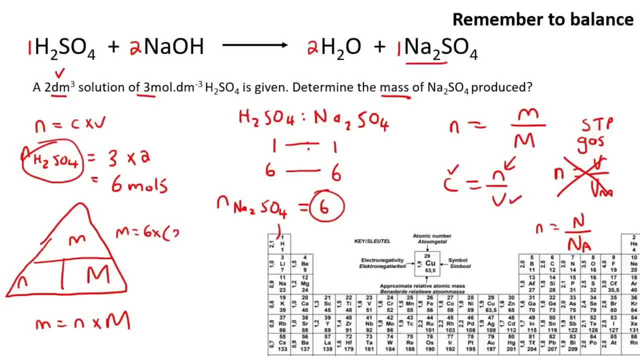 m is equal to six multiplied, so two sodiums, that's going to be 2 times 23, plus it's got one sulfur. now each sulfur has a mass of 32 plus and then four oxygens, so that's going to be each one has a mass of 16.. if you had to go calculate this, you get a big mass of 800. 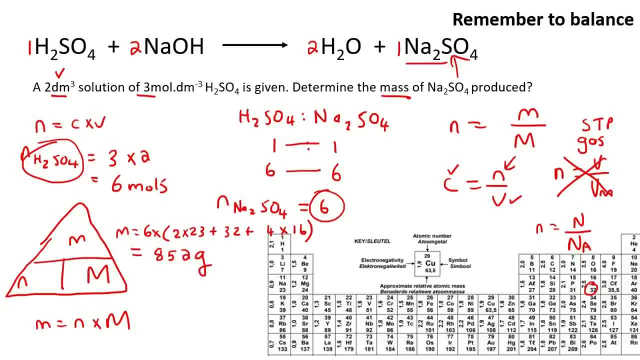 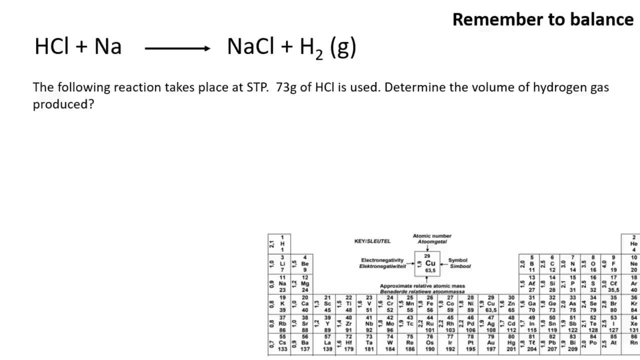 whoopsie 852 grams. so here's our next question. so the first step is always to balance. okay, so the way we balance is we use these steps over here. so we we divide our reaction into two halves: the ones stuff on the left and the stuff on the right of the arrow. so on the left we have 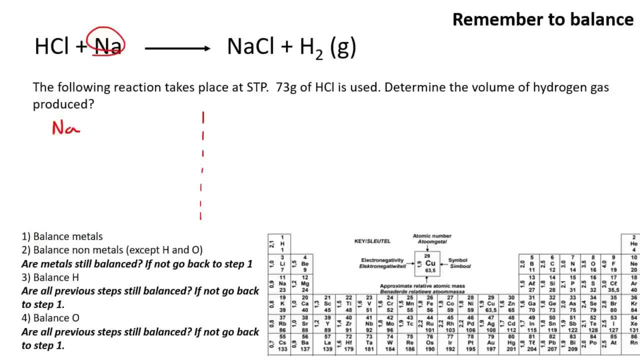 na, which is a metal? okay, because it says: balance all the metals first. so on the left we have one and on the right we also have one, so those are balanced. so now we go balance all of the non-metals, except for things like hydrogen and oxygen. so that would be a non-metal, would be. 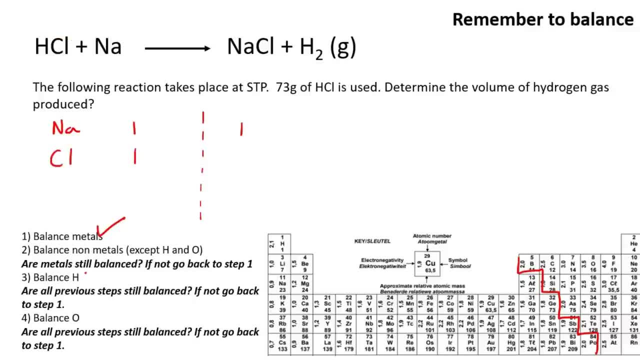 cl. so on the left we have one and on the right we have one. so that's good. now we go balance all of the hydrogen, okay. so on the left we have one and on the right we have two. okay, so we need to fix that. the way that we fix that is we put a two in the front here, but now that two has now made 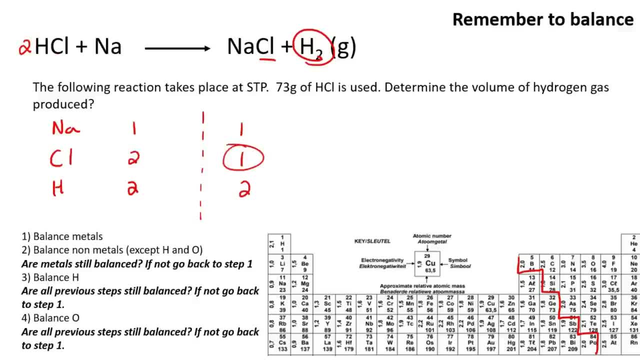 two cls. so now we have two cls on the left, so these aren't balanced anymore. so to fix that you have to change the cl to a two. but you can't put a two there because those valency numbers are already balanced. do you put it there, and so there we have it. but now, by putting that two over there, you've now made two. 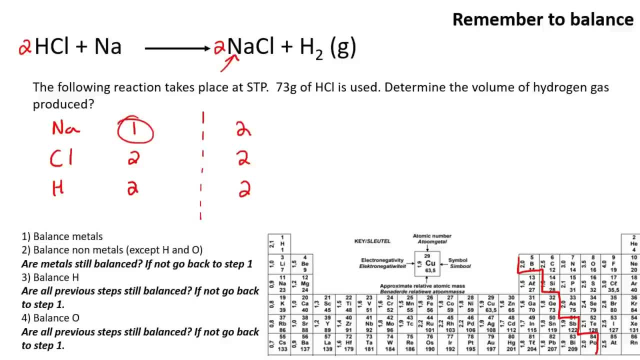 nas on the right, but look at this, there's only one on the left, so to fix that, we put a two in the front there. wow, this is actually an awesome one, and now everything is perfectly balanced. okay, now it is at this step where we can go and do the question. so they tell us that the following 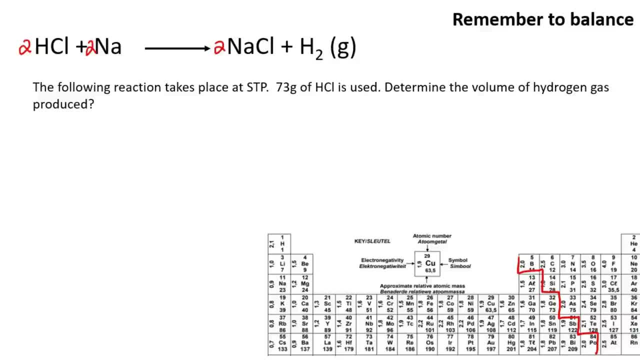 reaction takes place at stp. oh, did you see that stp? when you see that you should think about molar volume, which is something that only happens with gas, hello, which is going to be a number, 22.4 decimeters- okay, they'll give you this in the exam. uh, on your, on your um formula sheet, for example. 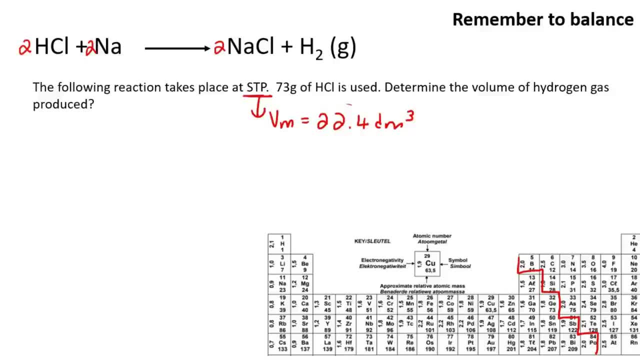 okay, so we know that we are busy with a gas. we can use a certain formula. so they tell us that 73 grams of hcl is used. okay, now we've got these different formulas. uh, this one, we've got this one, and we've got this one now. this question doesn't talk about 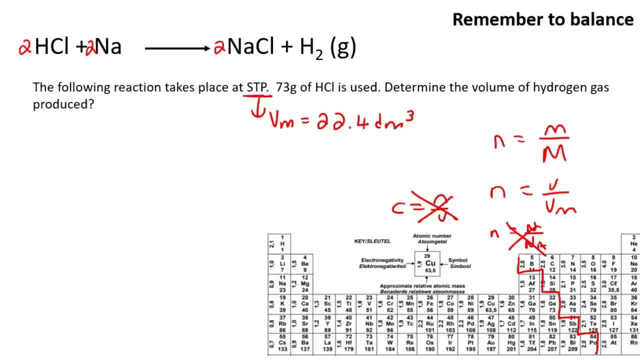 concentrations or number of particles. so we're going to start with the hcl. okay, now they give us the mass, so we're going to use this one for hcl. so let's go calculate that first. so it's going to be equal to its mass divided by its molar mass. now, remember, the molar mass is on the periodic table. 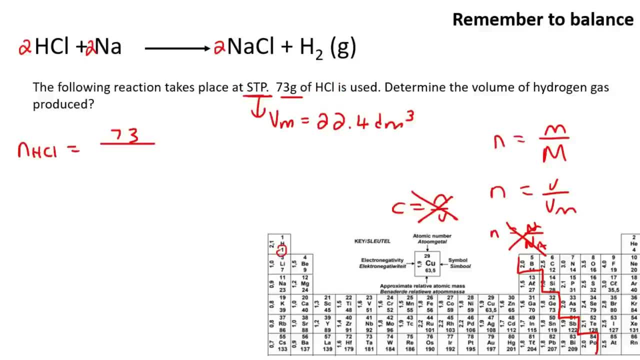 so hcl. so that's going to have one hydrogen and then one chlorine. now if you had to go calculate this, you end up with two mole, two mole. excellent. so we have the moles of hcl. once you have the moles of one of them, you can get the moles of any of the other ones. now they say: determine the. 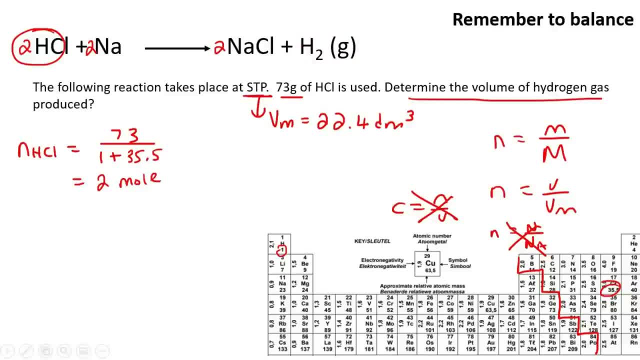 volume of hydrogen by the molar mass. so we have the moles of hcl and then we have the moles of hydrogen gas produced. okay, so they're talking about volume and they spoke about stp, so we can just use this formula, but we so, so so we're going to say n is equal to v over vm, so we know vm they. 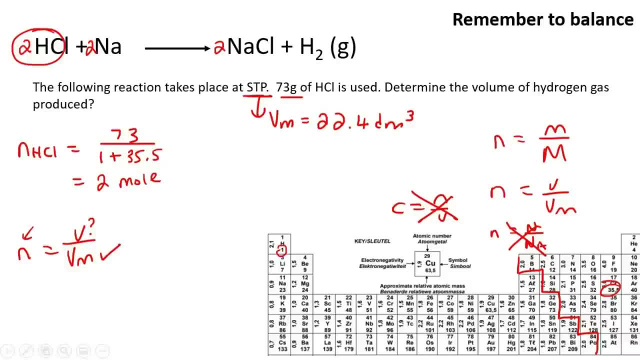 want us to calculate this, but we don't know the number of moles of hydrogen. we only have the moles of hcl. so here's where we use ratios. so we know that the ratio of hcl to hydrogen is a two to one. so two to one. so if we have two moles of hcl, we need to figure out how many moles of hydrogen. 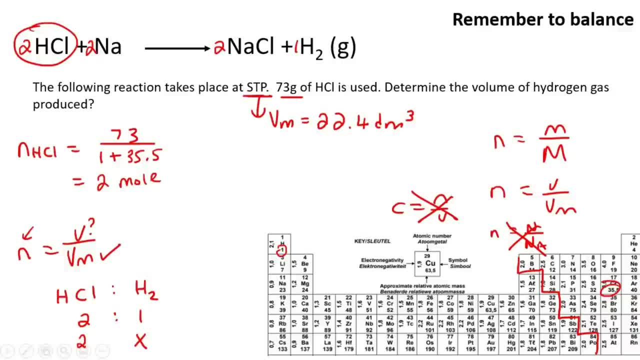 do we have now? some of you might be able to see the answer very quickly, but for those of you that are a bit confused, then what we do now, or what it means, is that for every- so for every two moles of hydrochloric acid, you're always going to have one mole of hydrogen. so this answer here for x is: 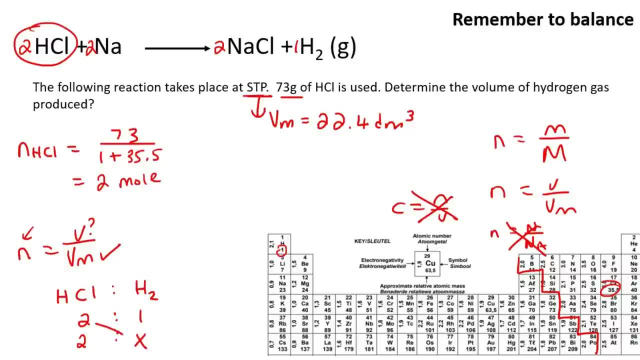 going to be a one, but let me just show you in case you didn't understand. so remember, i've showed you earlier in this lesson that what you do here is you multiply these two together, so that'll be 2x, and then you multiply these two together and that'll give you two. 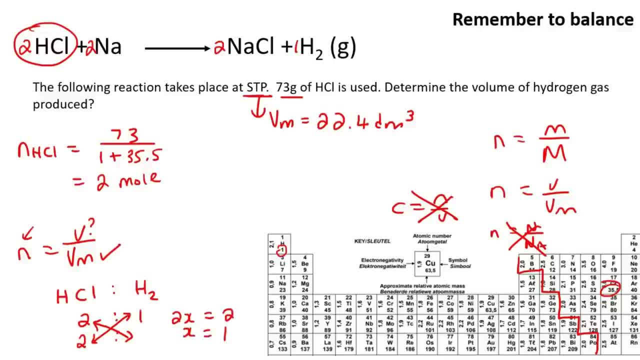 then you divide to get x by itself and x would be one. so the moles of hydrogen is going to be one, so the mole of hydrogen will be one. okay, so now we can use this formula, because now we have the number of moles and we have this. so to get this part by itself, you should have v. 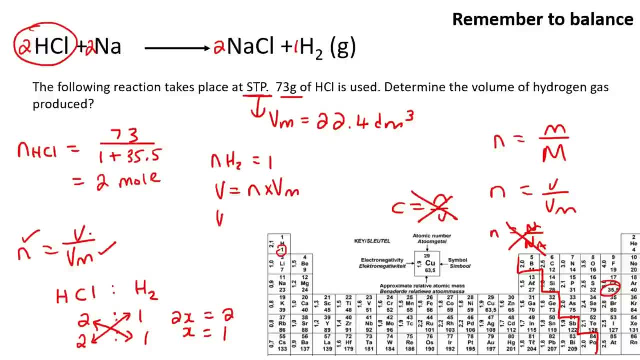 equals to n multiplied by molar volume, and so that's going to be one multiplied by molar volume, which is 22.4. kevin, where did you get that number from guys? that is a number that they will give you. it's a special number that i've spoken about where, if you are at stp- which is something i've spoken- 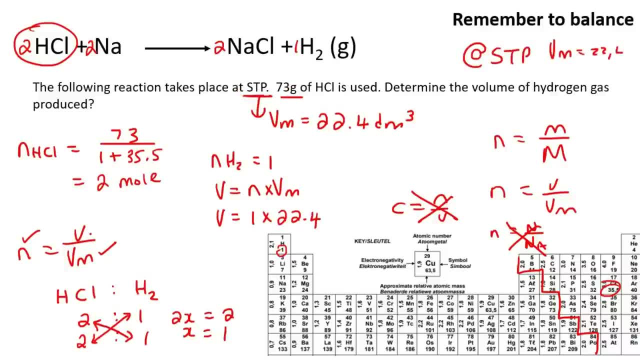 about before. then we can use vm as 22 comma 4, and so if you had to work this out, you would end up with 22 comma 4. let's just write it a little bit better. you'd get 22 comma 4 decimeters.